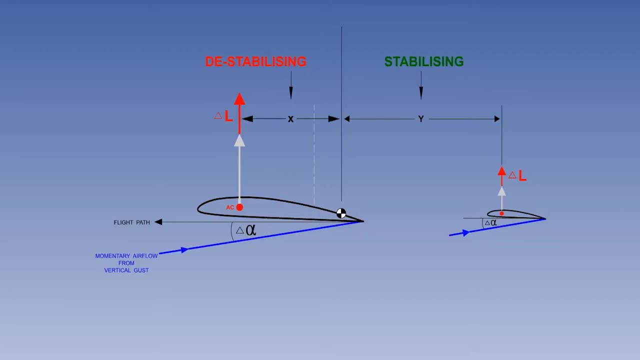 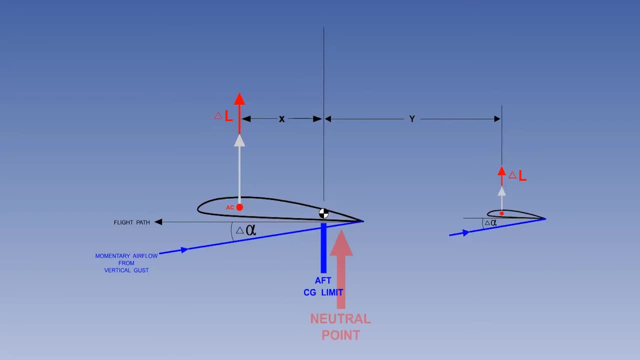 Calculating the CG position during the entire flight will be fully covered in a different subject called mass and balance. If we now move the CG forwards of the aft CG limit, the longitudinal static stability will increase. But we don't want the CG too far forward. 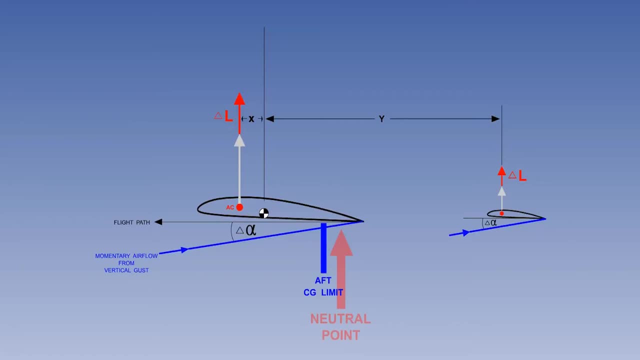 But we don't want the CG too far forward Because thereissuchathing, as two modes of motion, much longitudinal static stability. you might think the more longitudinal static stability the better. but no, in addition to our example gust, the pilot can also momentarily change the angle. 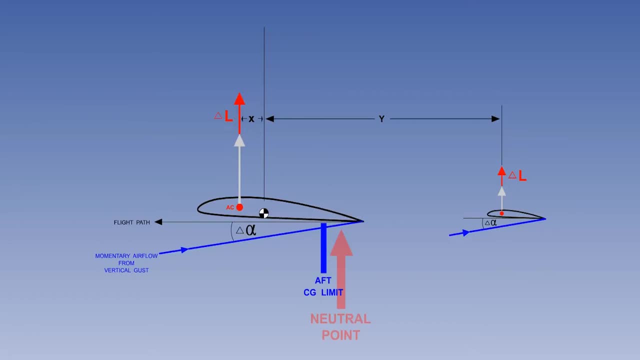 of attack when a pitch input is made. longitudinal static stability will oppose the pilots pitch input in the same way it opposes a gust. the greater the stability, the more the resistance to pitch input. so in addition to the effect of CG position on longitudinal static stability, we must also consider the effect of CG position on the ability of the pilot to maneuver the aircraft. 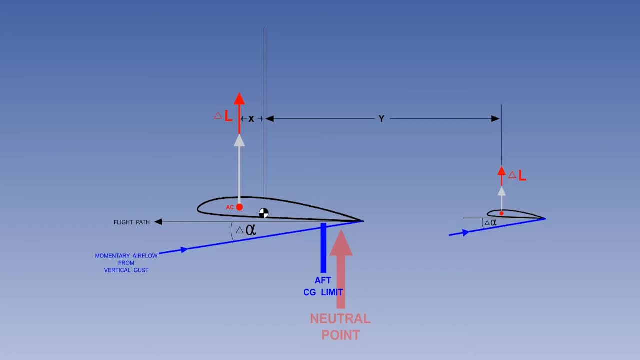 in pitch and the stick force is required. consequently, to ensure minimum ability for the pilot to maneuver the aircraft in pitch, plus ensure the stick forces are not too high, a forward CG limit is required. the forward CG limit will give maximum longitudinal static stability and guarantees minimum acceptable. 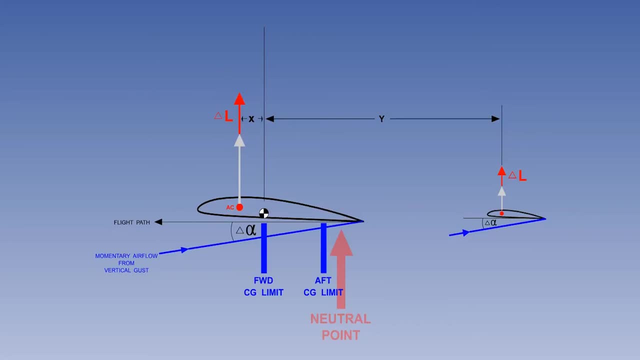 maneuverability and maximum acceptable stick forces. the aft CG limit will give minimum acceptable longitudinal static stability and gives maximum maneuverability and minimum acceptable stick forces. we will now take what we have learned about longitudinal static stability and organisations single sketch graphs. consider some of the variables. here are the two axes: the vertical axis represents pitching moment with increasing nose up pitching. 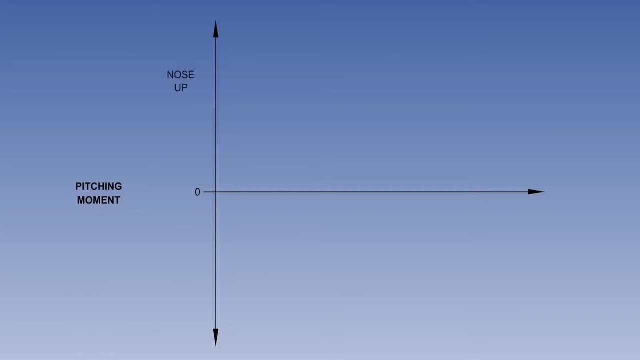 moment above the horizontal axis and increasing nose down. pitching moment below the horizontal axis is the pitching moment we know in machine learning the pitch moment is non-zero. tidal pitch in the vertical axis is the pitch moment and this means that the pitch is not perfectly paralleled. so the vertical axis is shorter than the horizontal axis on the tiered 걸. ie in combines order. 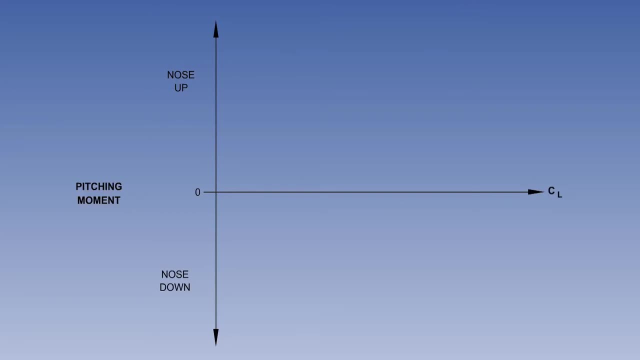 less computing ofaria lalous. a while below the horizontal axis it will become flammable shape possible. its triangle curve is the slope at which ilia зарready, thezentral square, is also called367 it is��이 axis represents lift coefficient increasing to the right. your previous 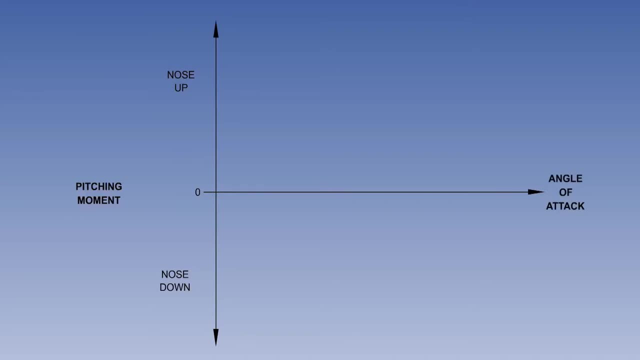 knowledge will tell you that the horizontal axis could instead be labeled angle of attack or decreasing indicated airspeed. as you will see, all three values need to be considered to give a full understanding of these graphs. for the time being, we will use lift coefficient for the horizontal axis, but 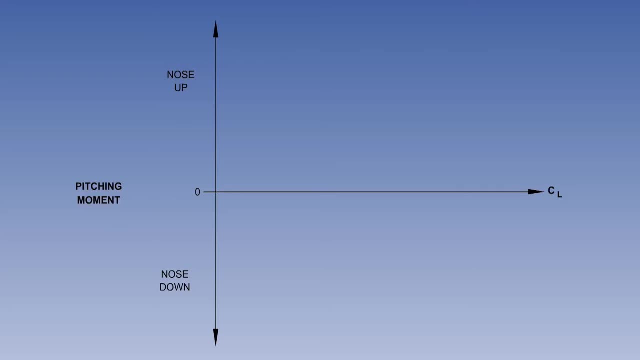 you need to keep the two alternative values in mind. an aeroplane in equilibrium is shown on the horizontal axis. how do we know it's in equilibrium? because it is not generating a nose up pitching moment or a nose down pitching moment. an upward acting gust has increased the lift. 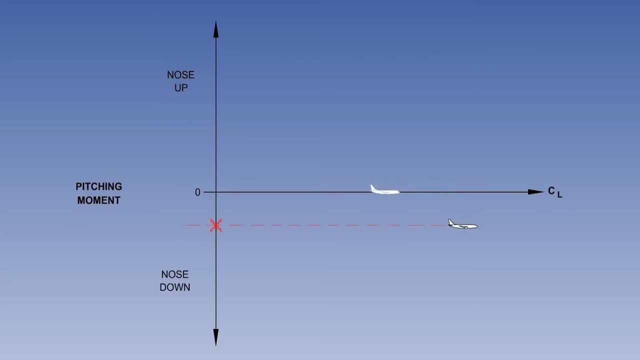 coefficient and because the aircraft has some longitudinal static stability, it will generate a nose down pitching moment. the nose down pitching moment will start the aircraft back towards equilibrium. remember, longitudinal static stability is just the initial reaction to a change in angle of attack. the graph is reset with the aircraft in equilibrium. 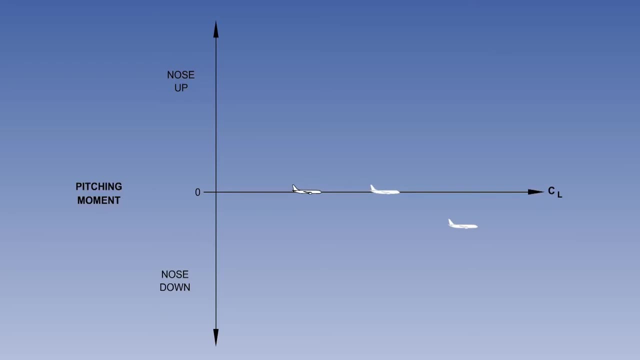 a downward acting gust now decreases the lift coefficient. because of its longitudinal static stability, the aircraft will once again generate a pitching moment, but this time it's a nose up pitching moment. the nose up pitching moment will start the aircraft back towards equilibrium. the graph is again reset with the aircraft in equilibrium. 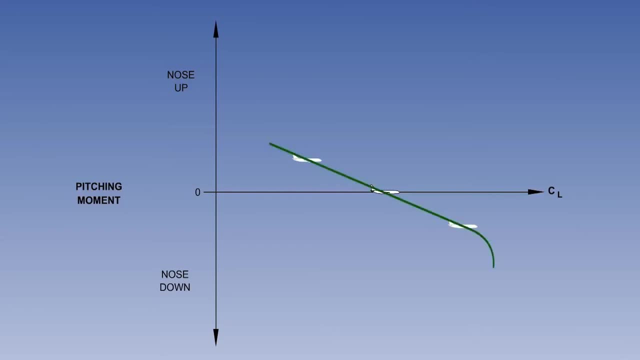 and if we join together the point on the graph that represents the aircraft in equilibrium, the point that represents the pitching moment generated by an increase in angle of attack and the point that represents the pitching moment generated by a decrease in angle of attack, the plot will represent a. 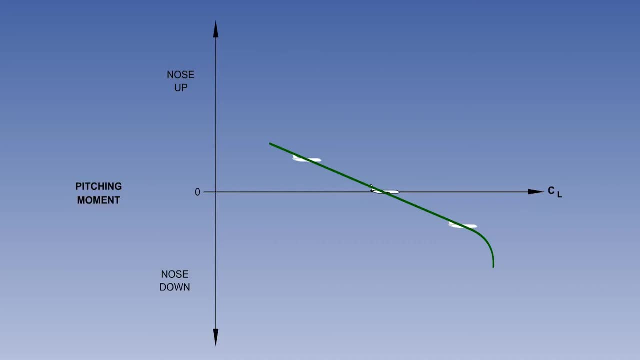 longitudinally statically stable aircraft. the curve on the right hand end of the plot shows the aircraft nose down pitching moment at the stall. now let's use the graph to consider variations in longitudinal static stability. movement of the red dot shows an increase in angle of attack, which generates a nose down pitching moment. 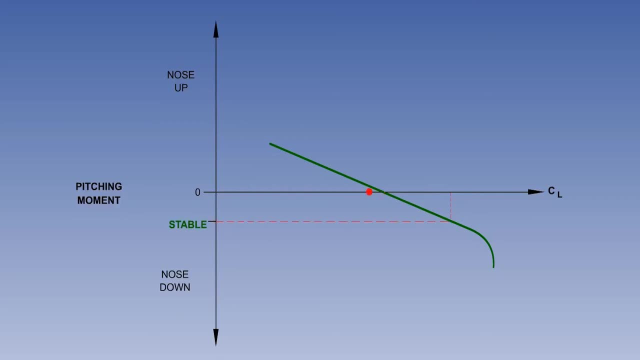 reset the graph to equilibrium. a decrease in angle of attack generates a nose up pitching moment. now we'll look at a decrease level of longitudinal static stability. the same increase in angle of attack has generated a smaller nose down pitching moment. reset the graph to equilibrium: the same decrease in angle of attack. 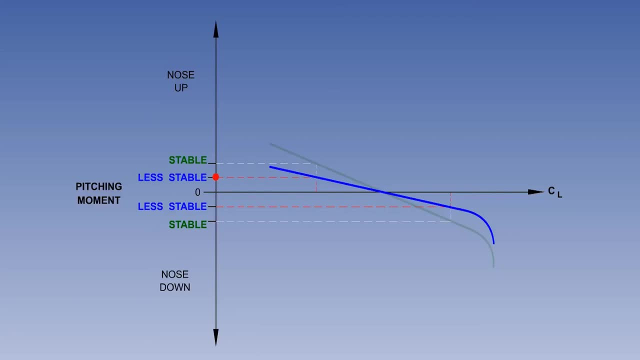 has also generated a smaller pitching moment, but this time nose up. the green plot shows longitudinal static stability. now we'll look at an increase level of longitudinal static stability. the same increase in angle of attack has generated a much bigger nose down pitching moment. reset the graph to equilibrium. 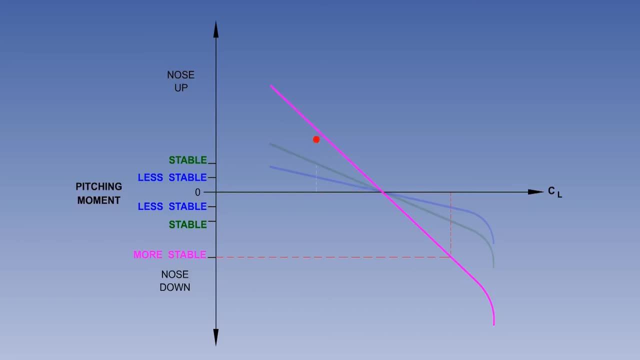 the same decrease in angle of attack has also generated a much bigger pitching moment, but this time nose up. the green plot shows longitudinal static stability. the blue plot shows less longitudinal static stability. the magenta plot shows more longitudinal static stability. the direction of all three plots is downward, from left to right. 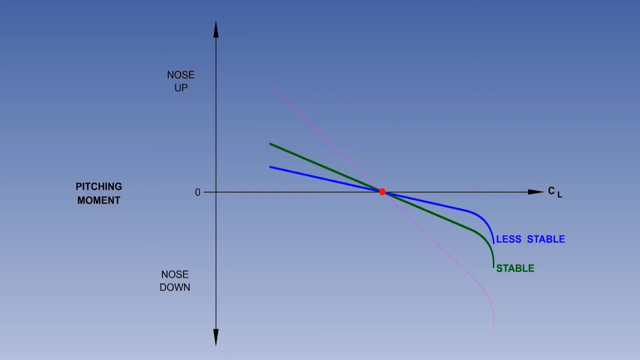 this indicates positive longitudinal static stability. the angles of the plots shows the amount of longitudinal static stability. the horizontal of the plots is the same as the horizontal of the plots. the horizontal of the plots is the same as the horizontal of the plots. the horizontal of the plots is the same as the horizontal of the plots. 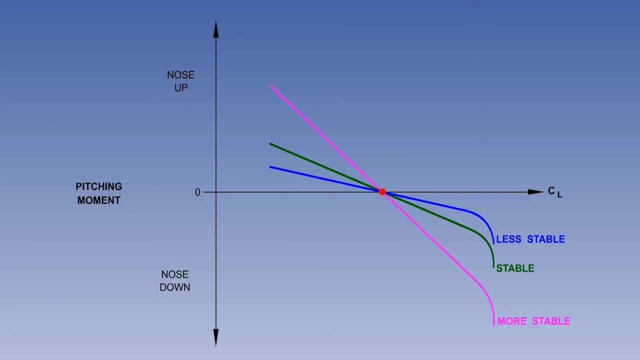 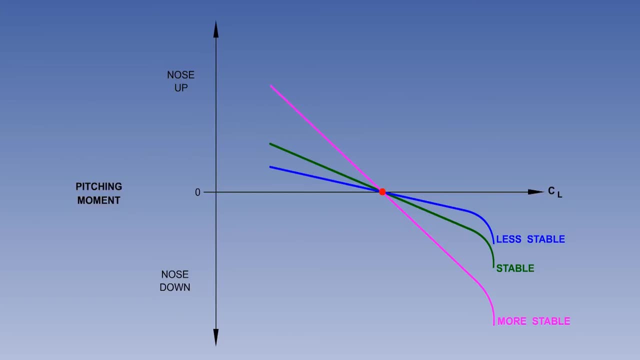 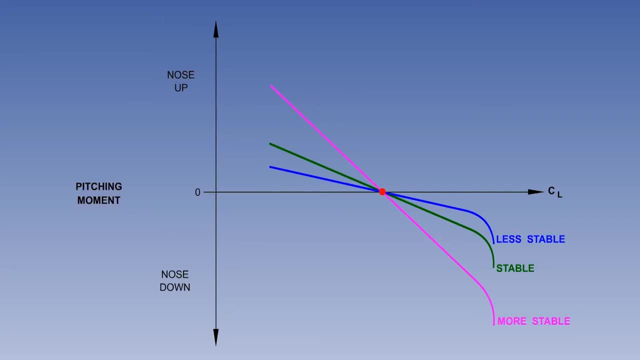 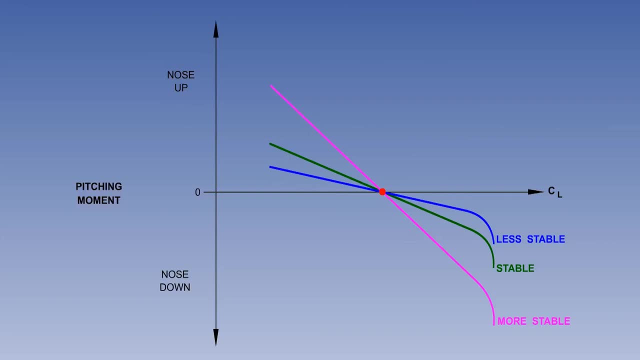 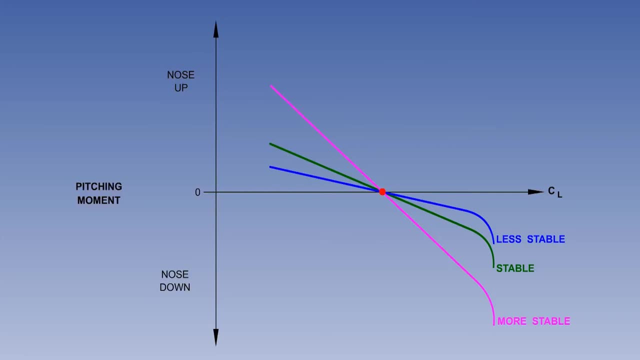 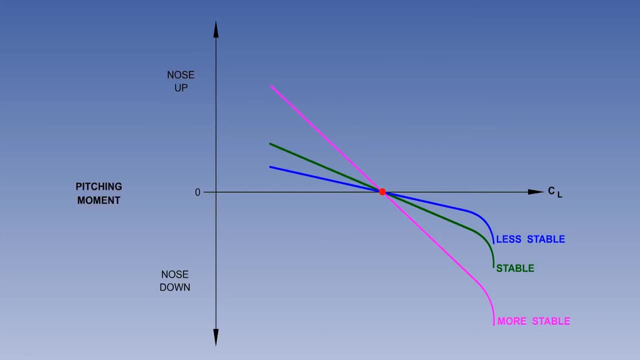 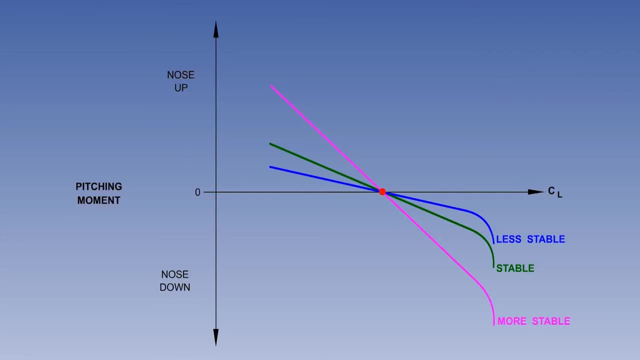 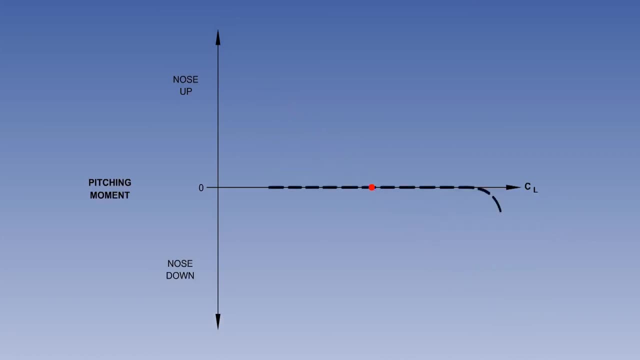 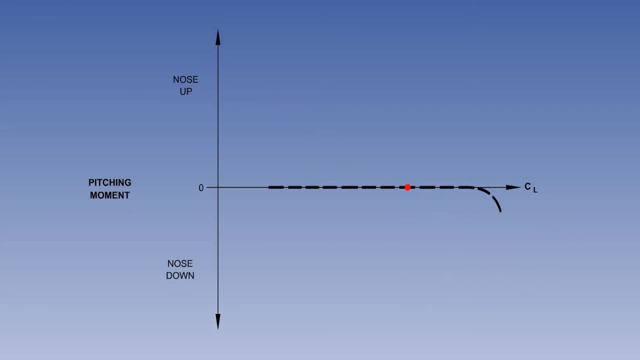 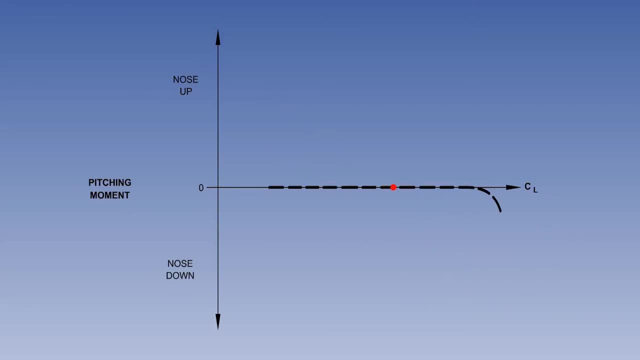 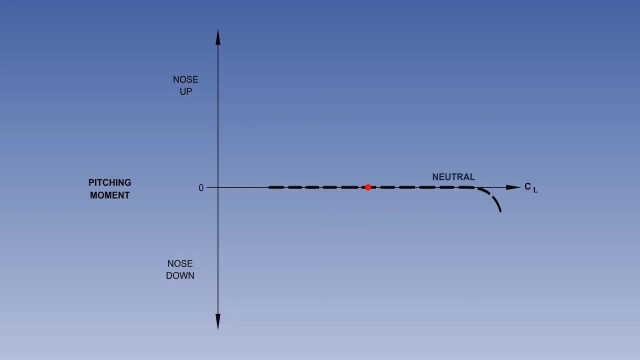 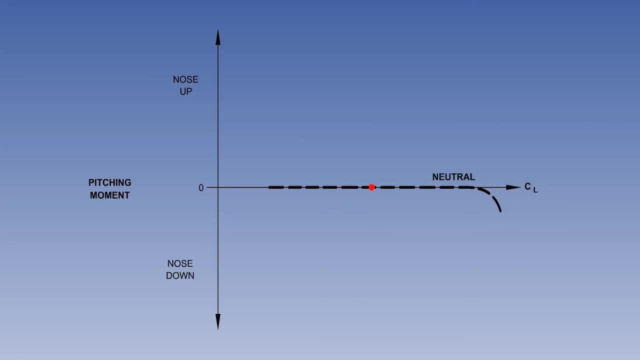 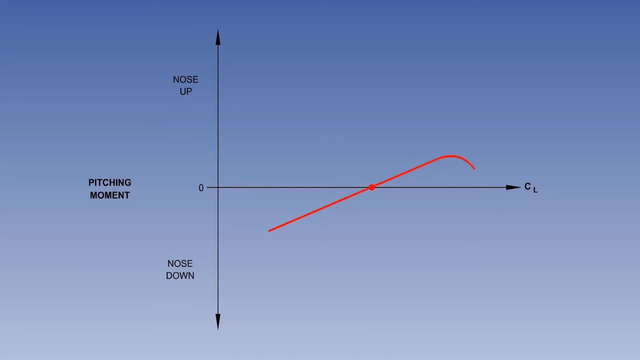 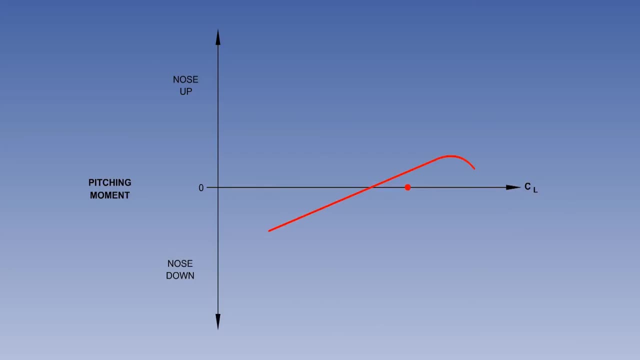 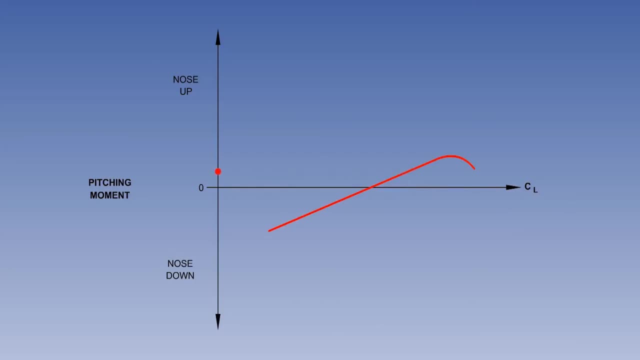 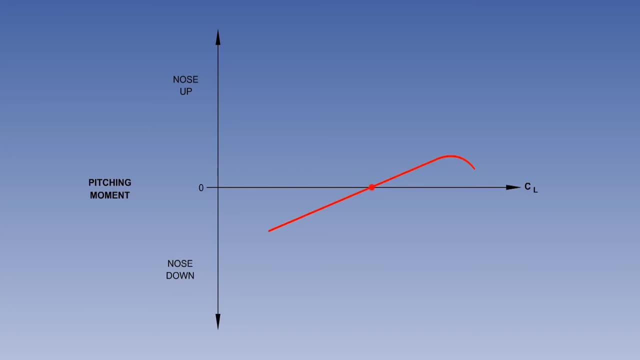 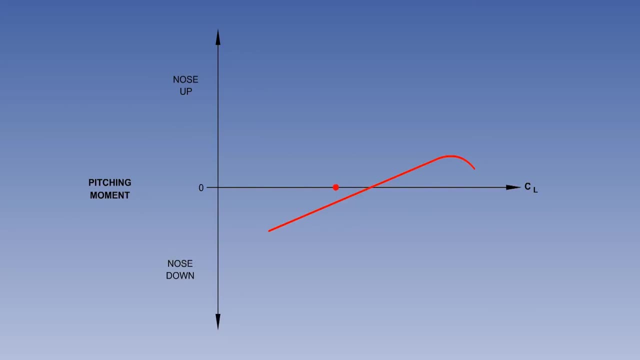 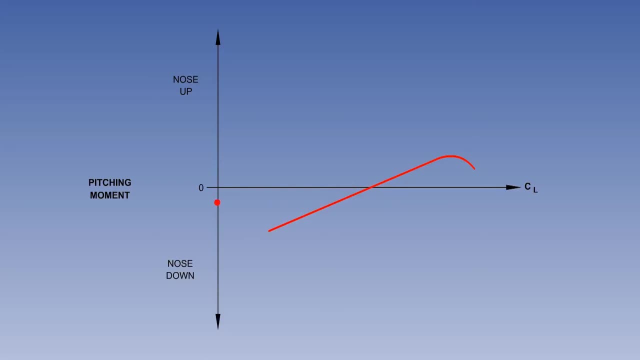 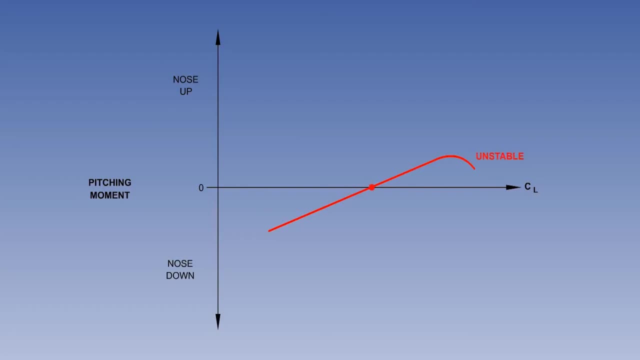 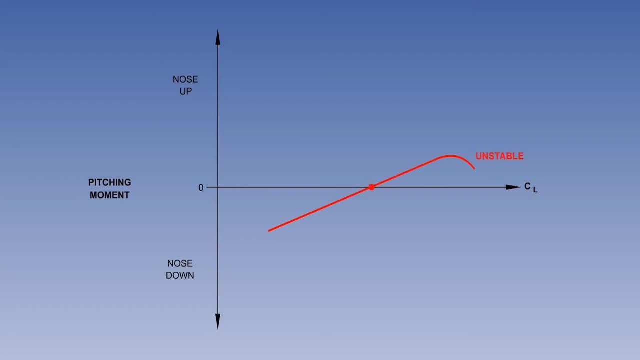 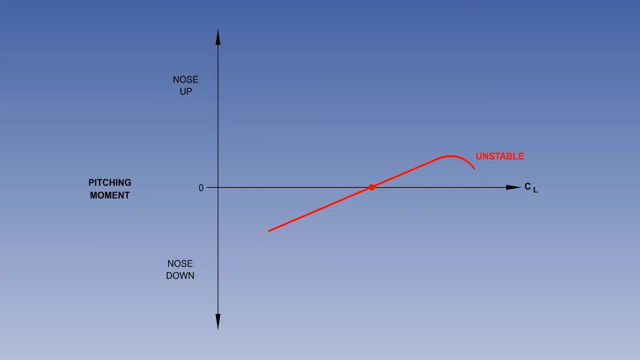 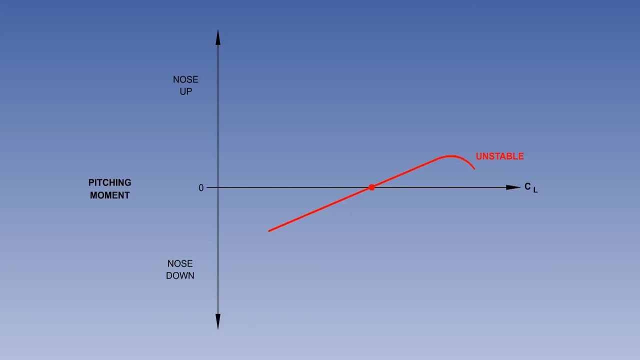 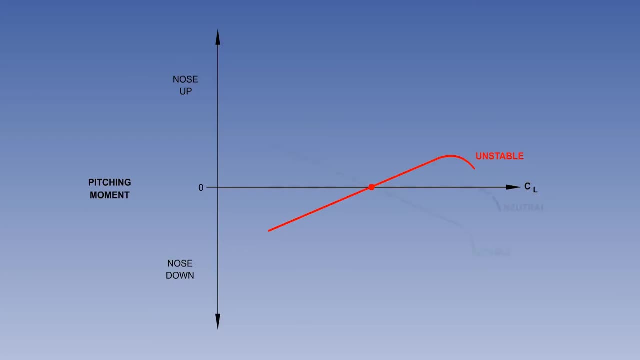 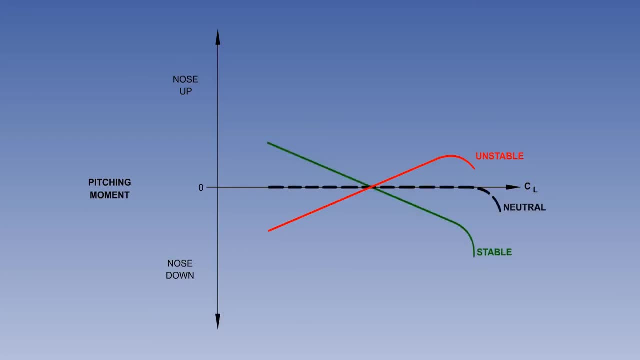 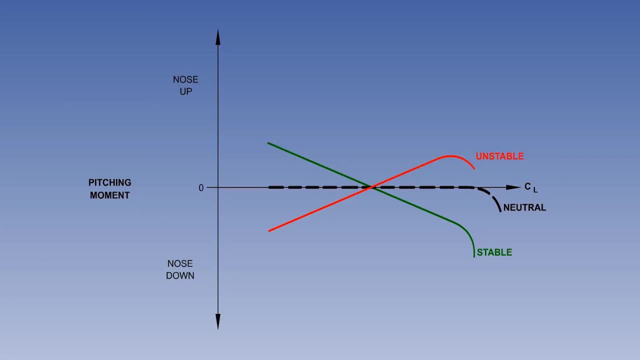 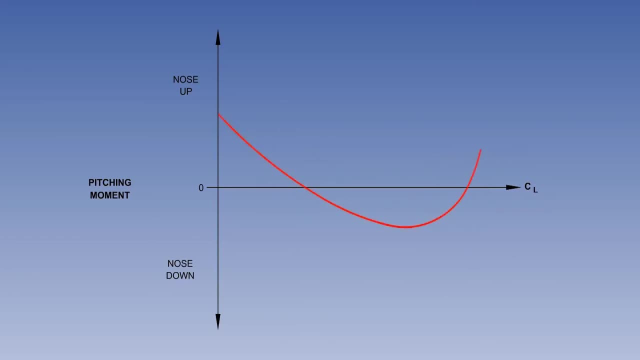 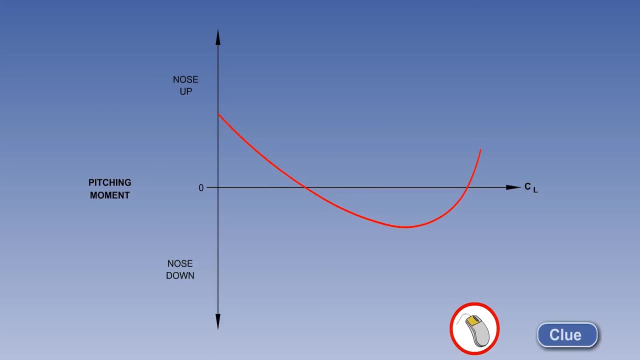 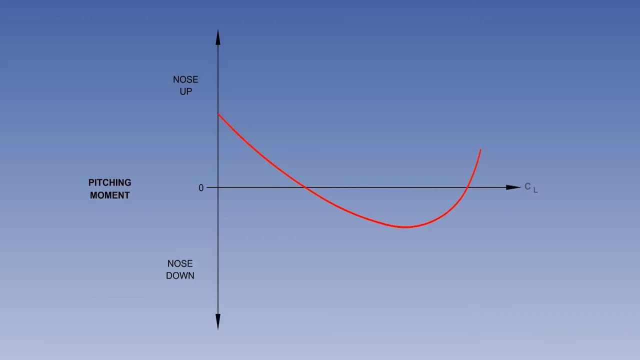 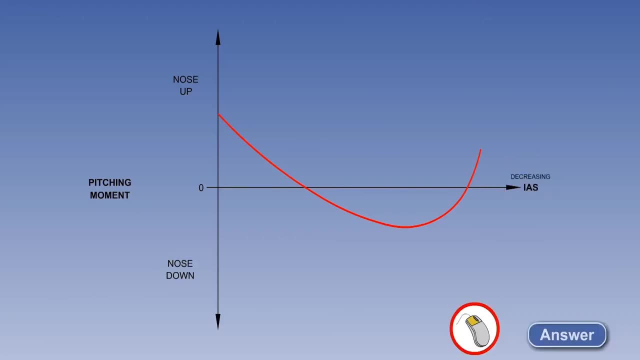 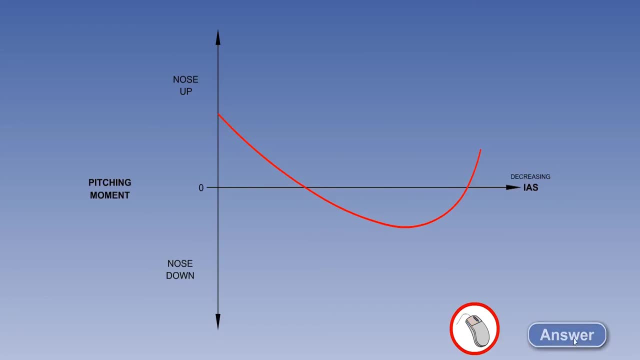 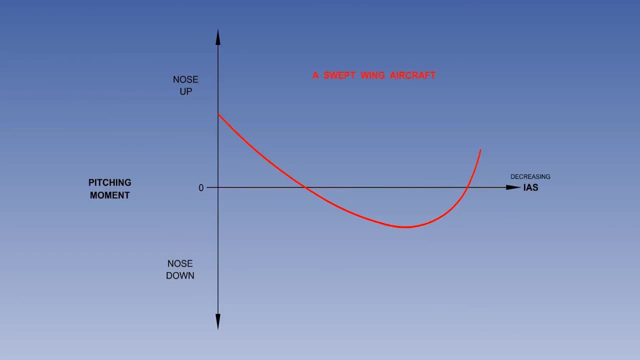 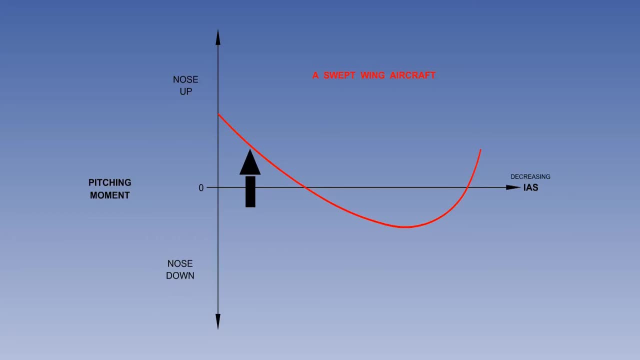 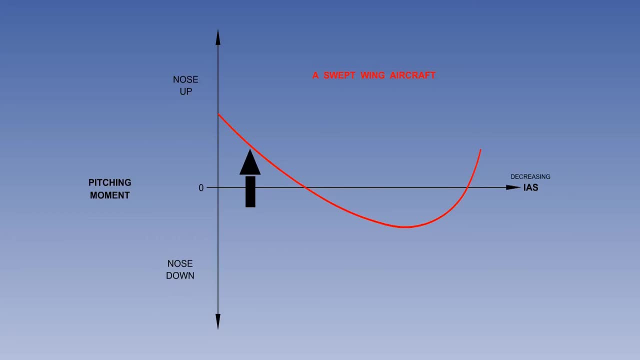 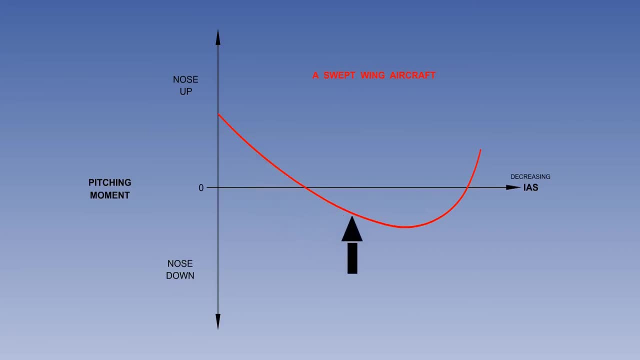 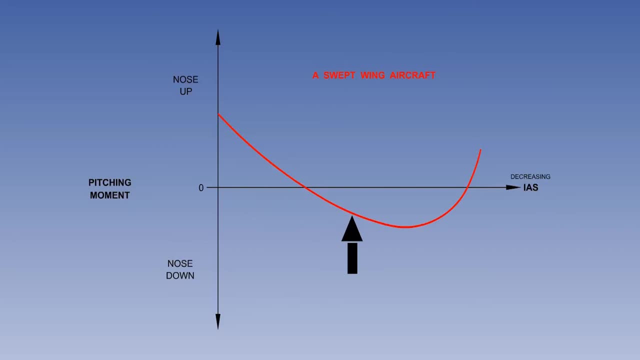 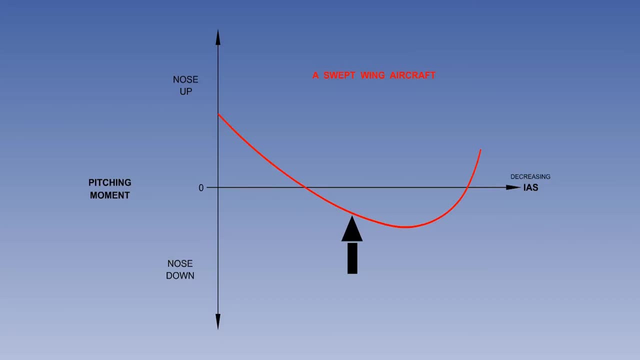 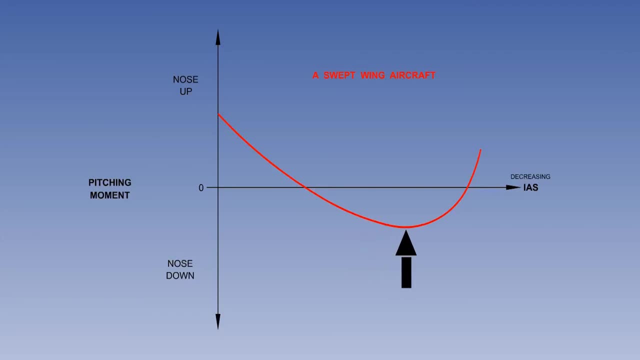 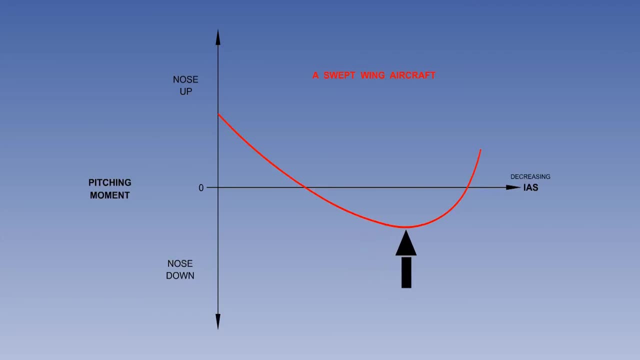 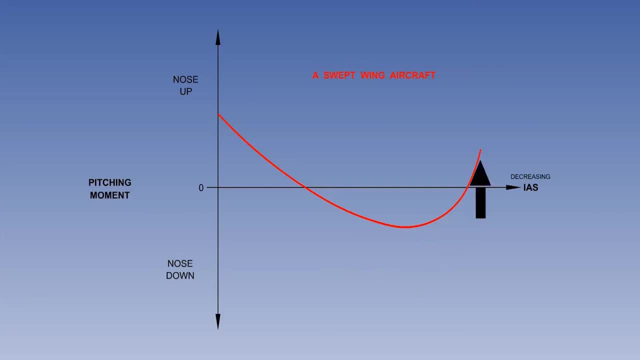 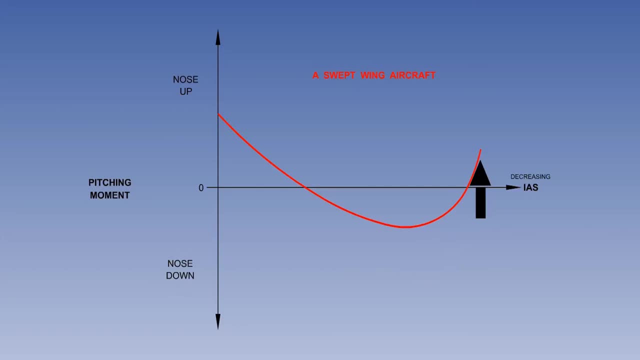 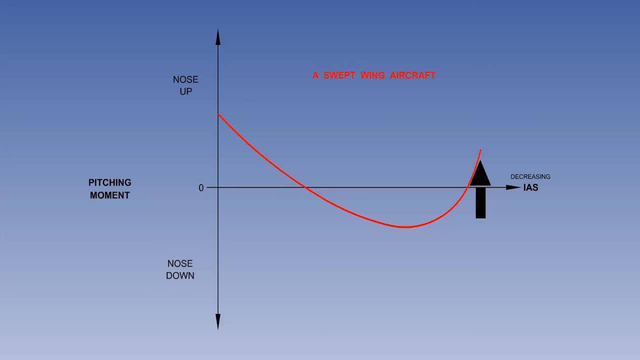 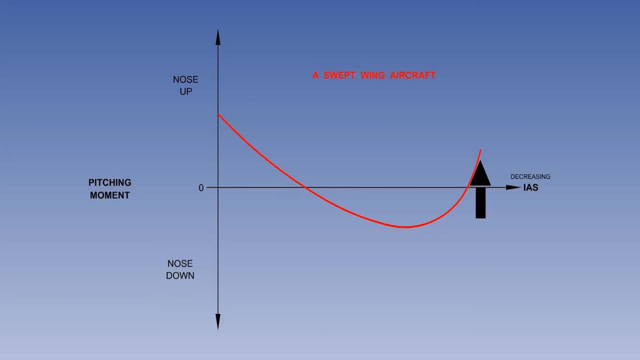 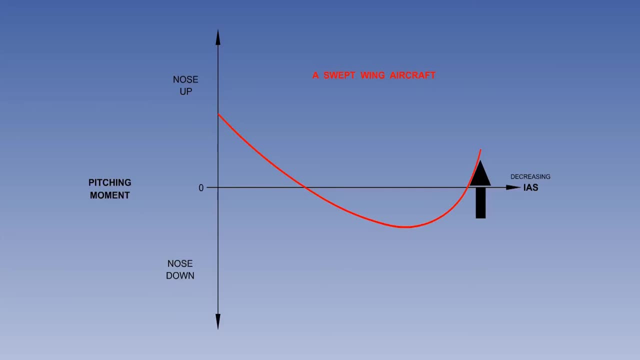 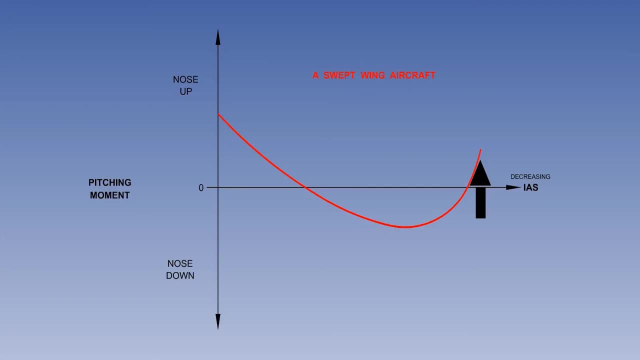 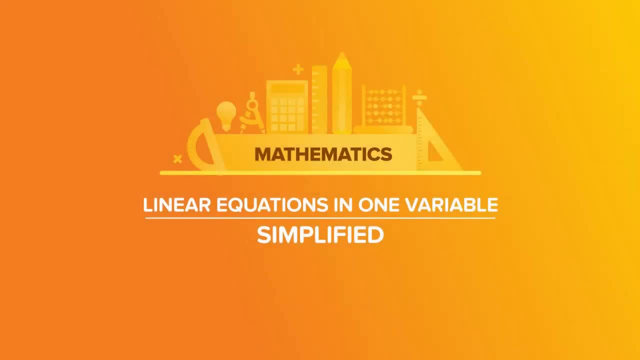 Linear equations in one variable. That's our topic for today. Lot of big words there. Linear, equation, variable. Let's see if we can understand all of these. Let's start with equation. So what 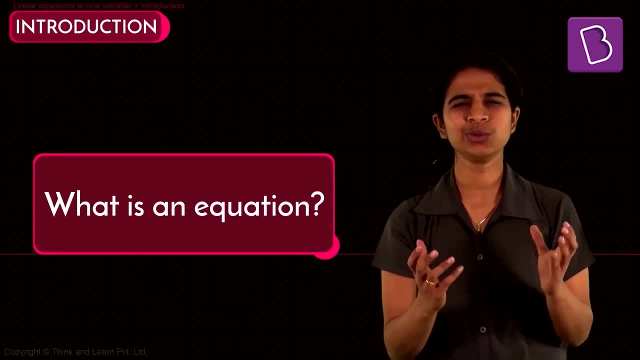 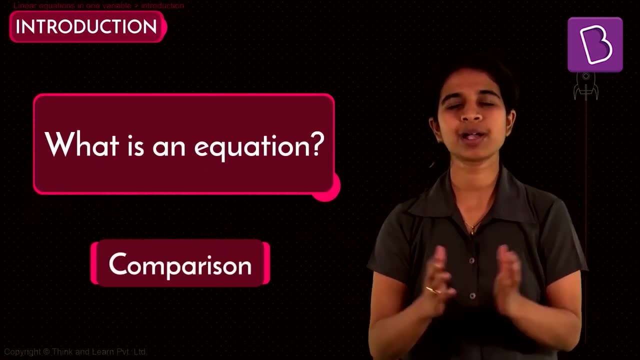 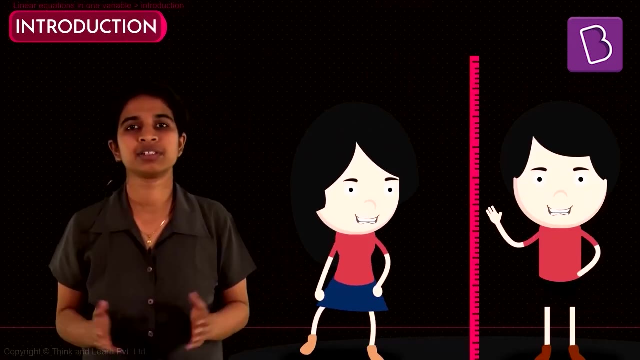 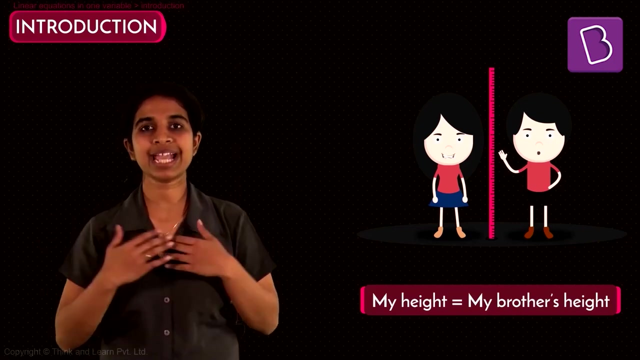 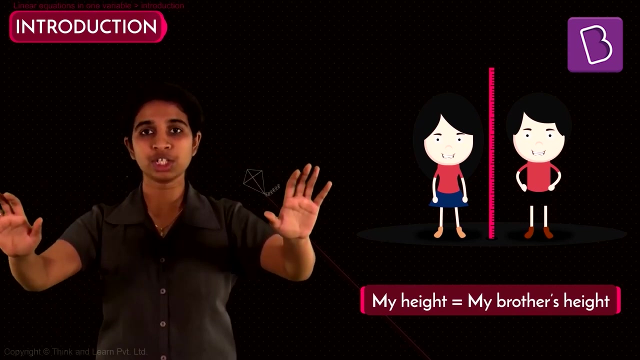 is an equation? Equation, equal to, looks like something like equal, right? What is an equation? In very simple words, an equation is nothing but a comparison. This is equal to this. Both of these are exactly the same. I am as tall as my brother. How could you write it as a mathematical equation? My height equal to my brother's height. That is nothing but saying I'm as tall as my brother. This is nothing but an equation. What it tells you is there's an equal to sign in between. And what is on the two sides of it is exactly the same. So my height and my brother's height is exactly the same. So my height and my brother's height is exactly the same. 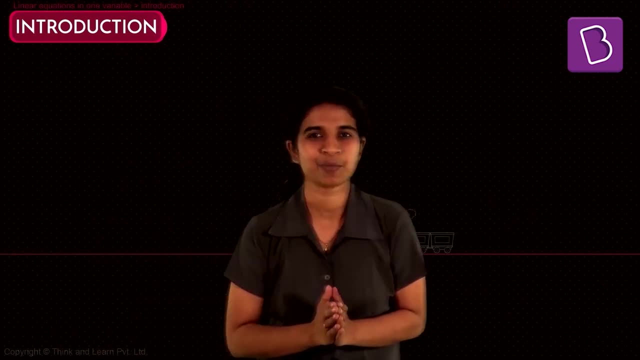 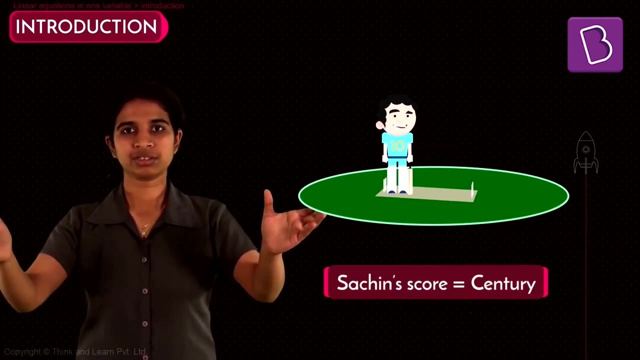 That's what an equation tells you. Now if I tell you such and scored a century, how do you write that? Such and scored is equal to a century. Or such and scored equal to 100 runs. 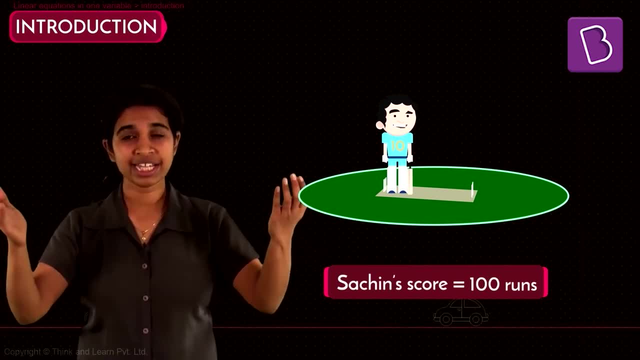 That is such and scored and 100 runs. Or such and scored and a century is one and the same thing.